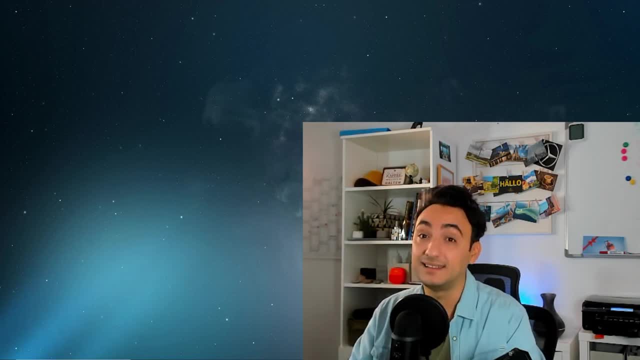 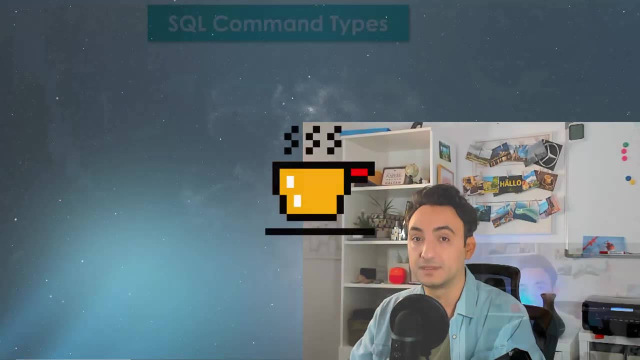 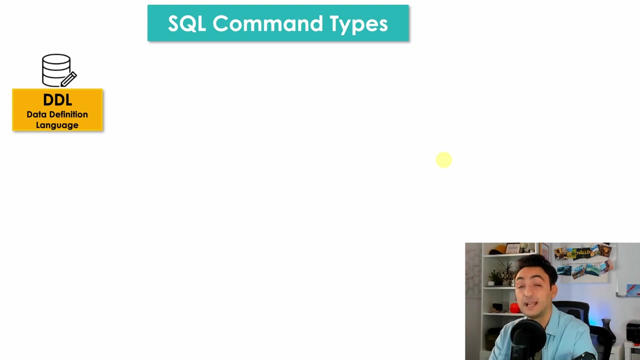 that I use in my projects in the last 10 years To make our life easier. SQL commands are divided into different groups depending on their purposes. All right, let's start with the first group: Data Definition Language- DDL, As the name suggests. here you will find all the commands that 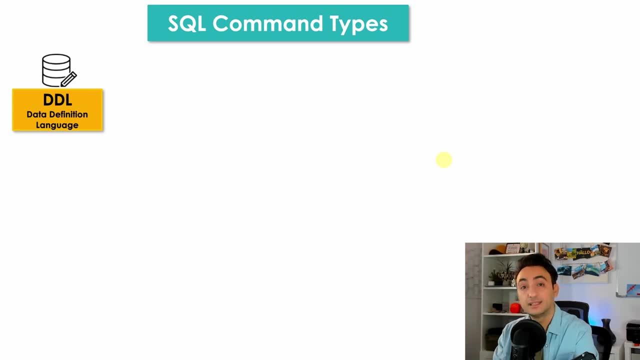 allow you to define your database, like creating tables, dropping columns, changing tables- anything that's going to change the structure of your database. Underneath this group you can find commands like create, which helps you to create anything new in the database. like create. 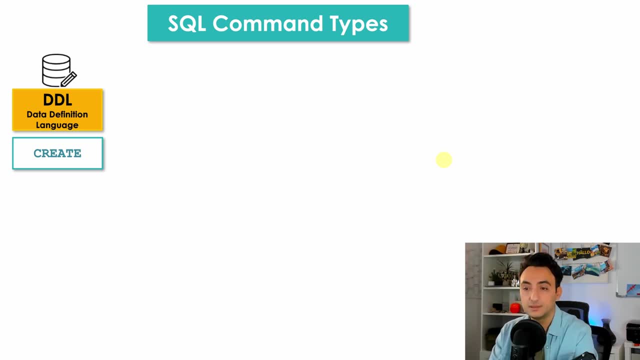 new tables, Create new views, store procedures and so on. One more: we have here the drop commands that allow you to delete one object from your database And the last one, alter. It helps you to edit the structure of your database, like altering one table, to change a column or to add. 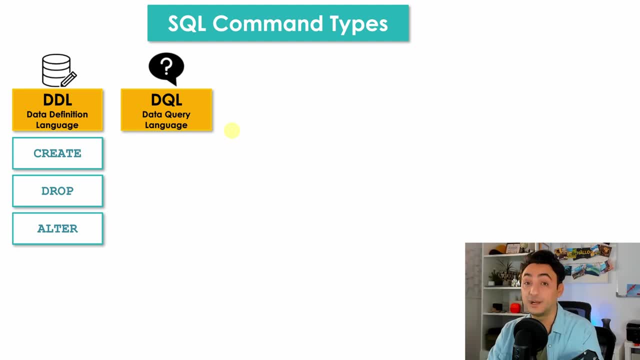 a new column. Okay, so now to the second group. we have Data Query Language, DQL. It contains only one command and that's enough. It's called the select command. It helps you to retrieve your data from your database. Select is the most important command. 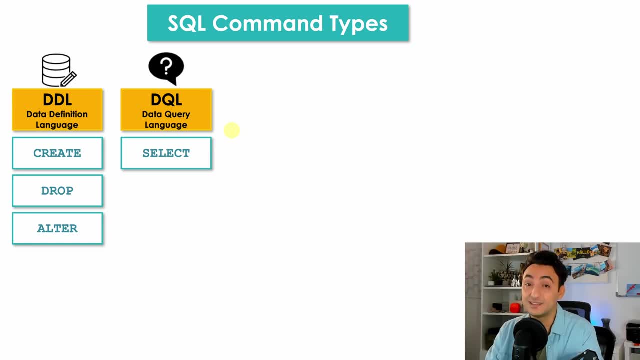 that we have in SQL and the one that you need to master in order to be good in SQL. In my tutorials, I will be explaining everything about the SQL select statements, because if you start working with SQL, you will end up writing tons of select statements, So don't worry about it. 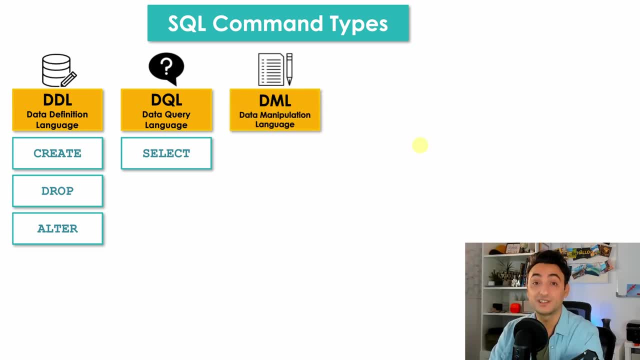 All right, let's go now to the next group. We have Data Manipulation Language, DML. DML contains all the SQL commands that you could use in order to manipulate your data inside your database. So we have commands like insert, in order to insert new data inside your tables. 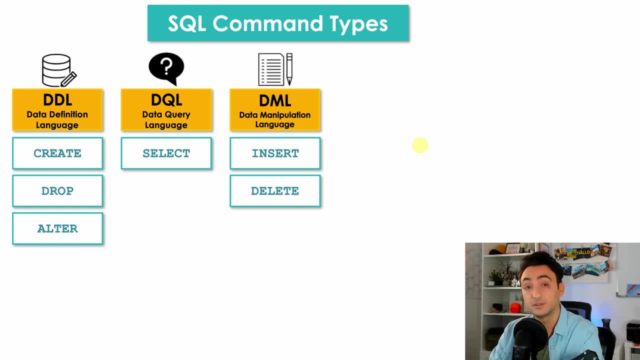 or we have delete to delete some data from your tables, or updates to update the content of existing data inside tables. So, as you see, it is really easy. The name tells everything. All right, so now we have two groups of commands. that is really more. 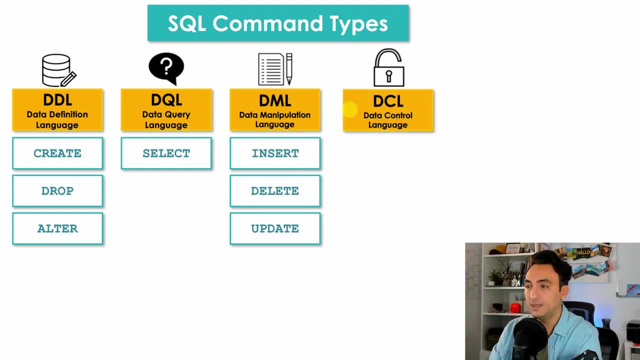 or SQL database administrators. So the next one: we have data control language, DCL. DCL contains SQL commands that allows you to give access to specific user to your database or to tables or schemas and so on. So here we have two commands: grants: you could use grants to give. 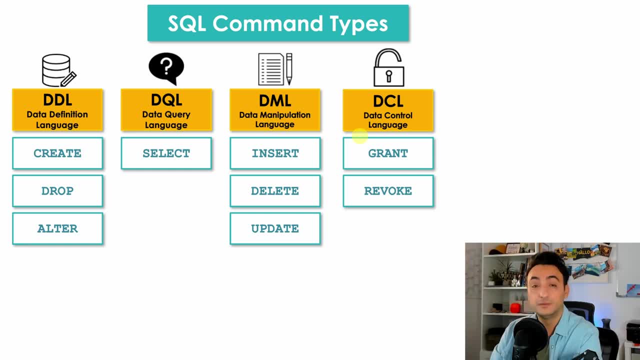 someone an access to your objects in databases or revoke to remove such access from specific user. Okay, so now to the last group that we have And that's the Android database. So we have the Azure Окkit database. In the next group we have the database. Here you can see the database. 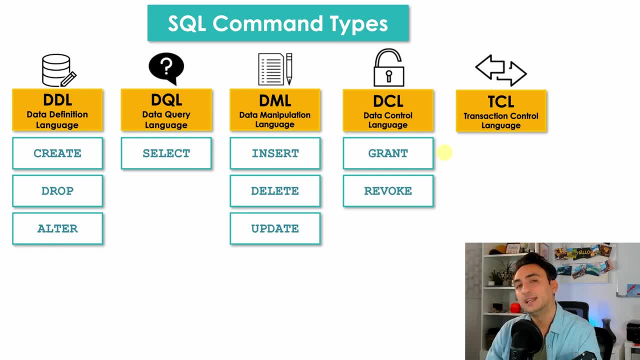 You can see the database itself And this database- I just put it in the description because it's also the database of any database- have the transaction control language, tcl. in tcl you will find the sql commands that's going to help you to manage the database transactions in order to maintain integrity of your data. 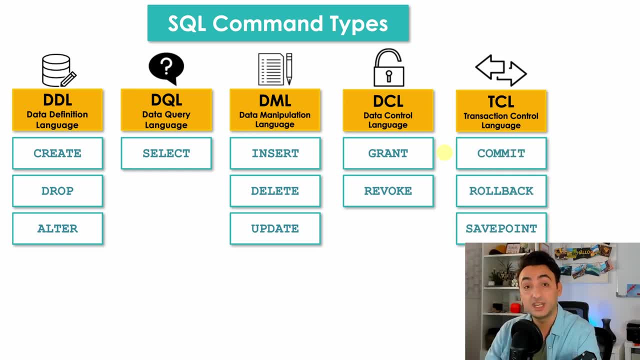 so here we have commands like commits in order to save the changes in your database. roll back to restore the database to the last commit or to the last save point. if you have some errors, you could use that save point. you can define save points in the transactions. 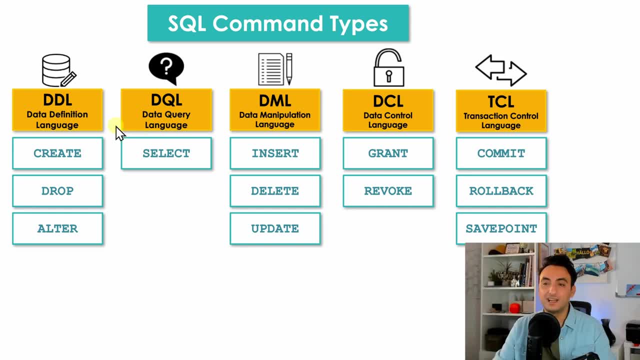 which you could use it later to roll back. alright, so now about those names: ddl, doql, dcl, tcl and so on, you don't have to memorize them. maybe only the important one is ddl. i sometimes hear it in the project, so if someone says i will be creating some ddl scripts, that means he or she can accrue it. sql statements to change the watermelon. while there's no argument sql script, there's no reason for it to need to fix it. it needs to be prepared for better insertion because so we have some methods that you can use in the transaction range. you might find good ideas. 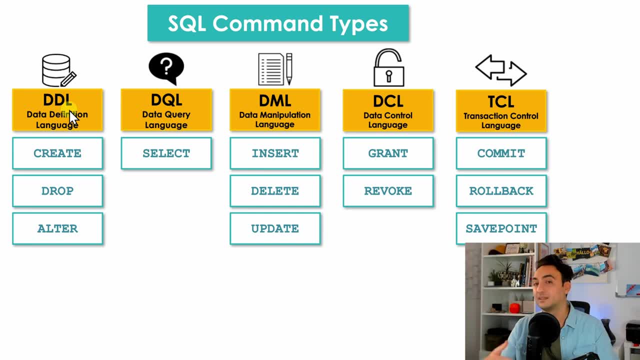 save point still needs to be provided, like a better upload is a standard running word and you can also have some errors. you could use those save point. you can define save points in the transactions which you can use it later to rollback, to change the structure of the database, like creating new table or dropping something all. 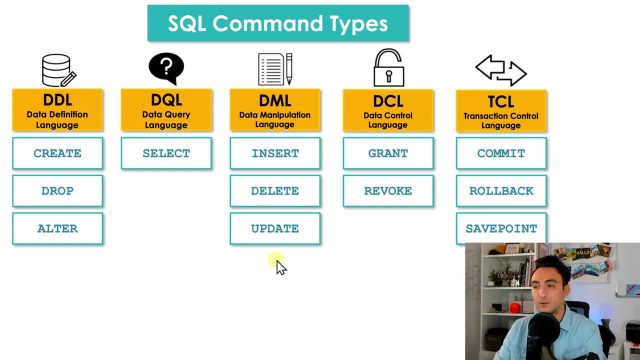 right. so in our sql tutorials we will be focusing on the first three groups of the sql commands. we will start with the most famous one, the sql select statements, and after that we're gonna deal with all those ddl scripts and finally i'm gonna explain insert, delete and updates. all right, so. 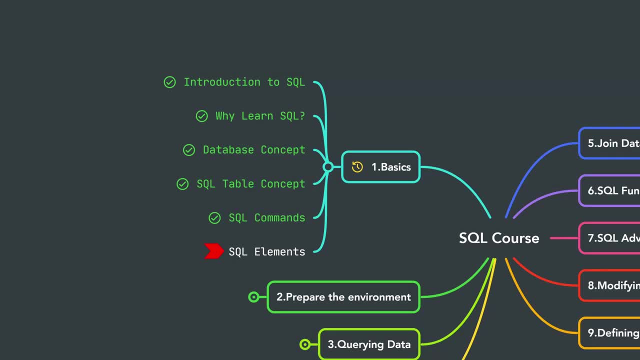 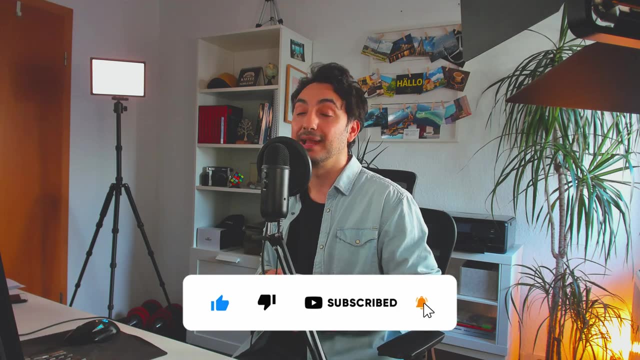 that was the main types of sql commands. next you will learn the basic elements of sql statements. and if you like this video and my work and you want to support the channel, then subscribe, like and comment, and in the video description you will find a link to free sql materials.